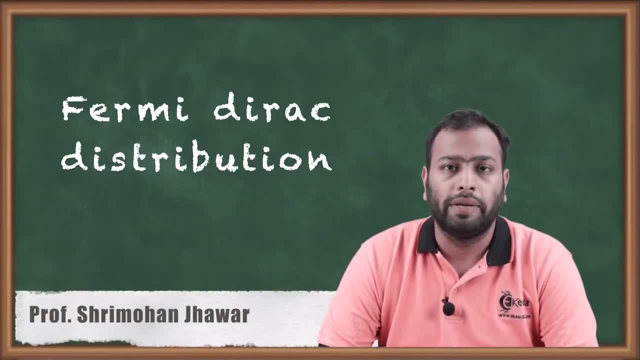 Hello friends, in today's class we will be studying about Fermi direct distribution. We had already studied about Fermi levels and Fermi energy in the previous classes, and now we will be extending our study towards Fermi direct function, which is nothing but. 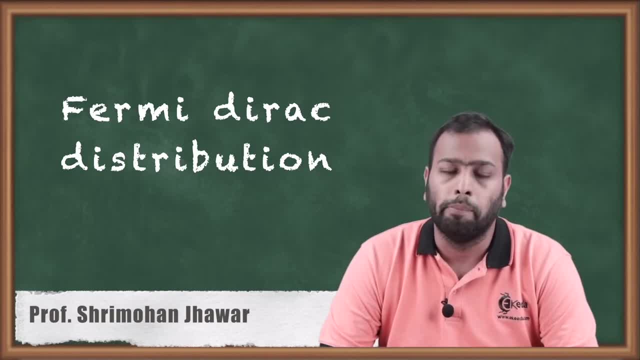 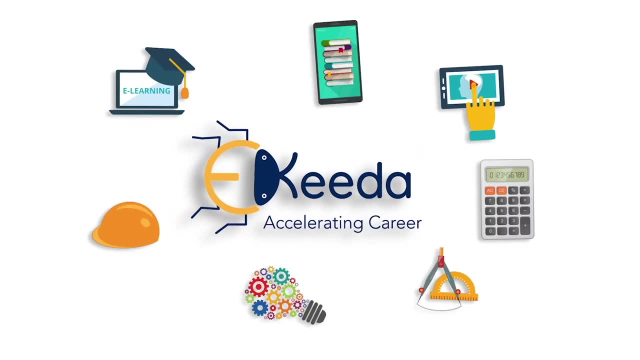 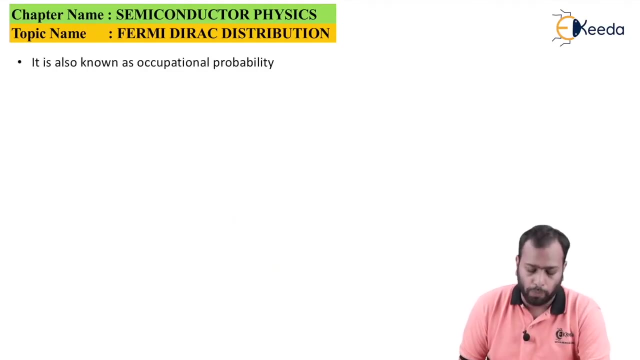 as the probability distribution function of finding an electron below and above the Fermi level. So let's begin. Fermi direct distribution is also known as the occupational probability. It is basically a probability distribution function which states the probability of finding an electron at a given energy level. As per quantum free electron theory, electrons are distributed. 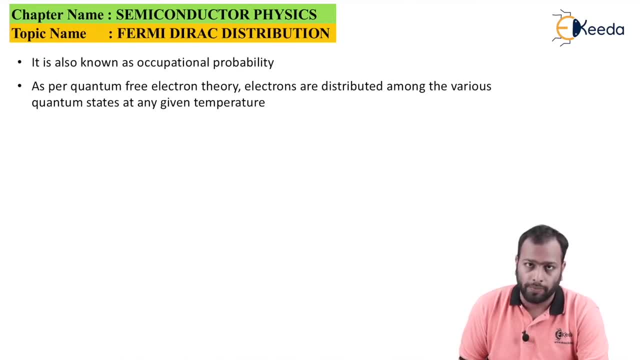 among the various quantum states at any given temperature. Well, let's first look at the probability distribution function of finding an electron. This means that if this is my energy state, E1, and this is the next energy state, E2, the electrons could be found at E1 or at E2, but it won't be found anywhere between Or you. 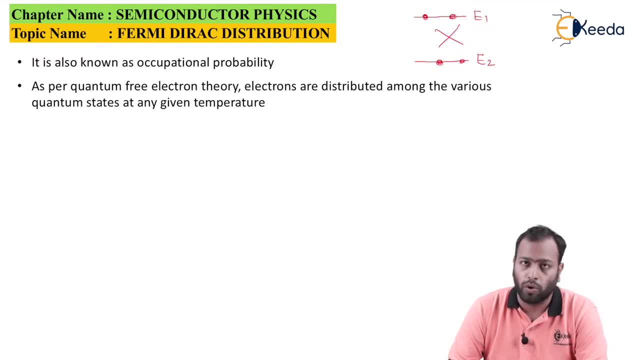 can say, electrons won't be present anywhere between the quantized energy states. Quantized energy states are the states which are fixed where the electrons will be found. The following considerations we have taken into picture while preparing the function of Fermi direct distribution. The first one is indistinguishability of the electron. Second, electron wave nature. 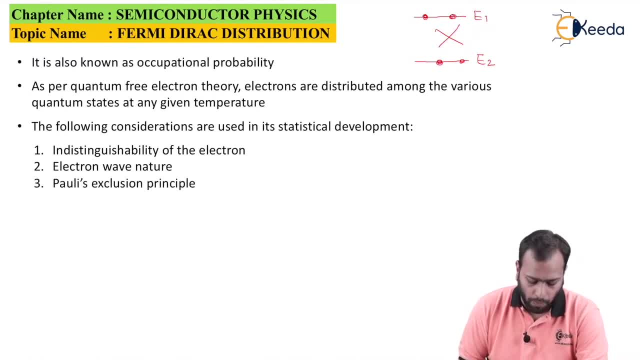 or the wave theory of the electron, And next is the Pauli's exclusion principle. Considering all the three factors, we have developed the probability distribution function, and this appears as: F of E equals 1 upon 1.0 to the power 3 times. And the first one is the probability. 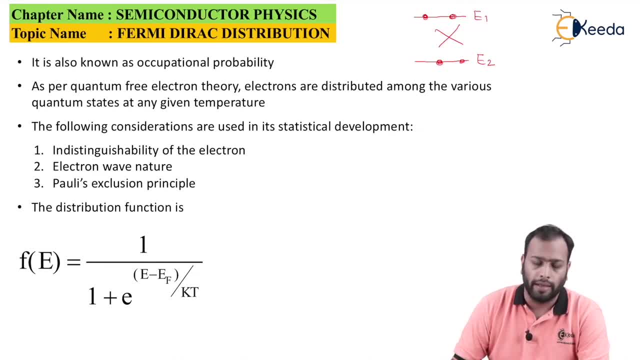 upon 1 plus e, raised to e minus cf over kt, Where f of e is nothing but is the probability that the electron with energy equal to e, Basically for any energy. if I want to find the probability, I'll be just plugging in the value for e and I'll be finding the probability of that electron. 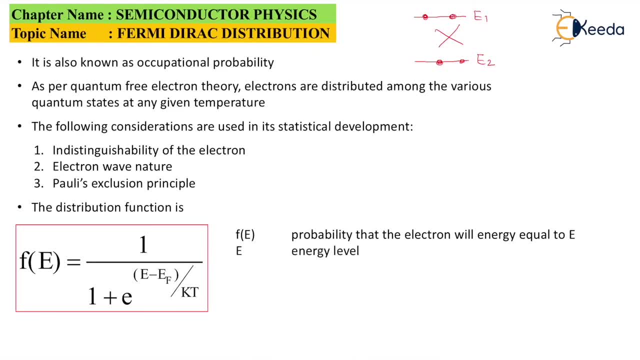 E is nothing but as energy level. ef is the Fermi energy, k is Boltzmann constant. You need to remember its value. Its value is 1.38 times 10 raised to power, minus 23 joules per kelvin. 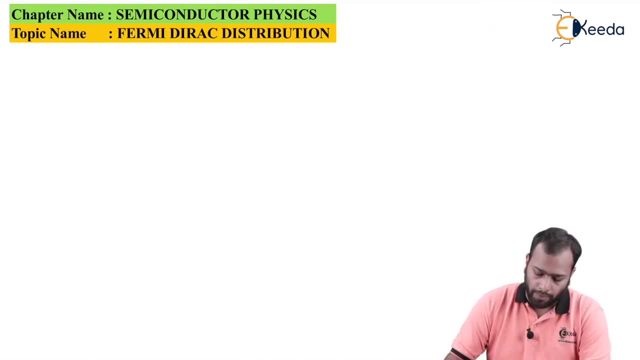 E is, of course, temperature in kelvin. Now let's take a case where t is equals to zero and e is less than ea. Now let's take a case where t is equal to zero and e is less than ea. Well, if e is less than ef, I can say e minus ef is less than zero, or I can say it is a negative. 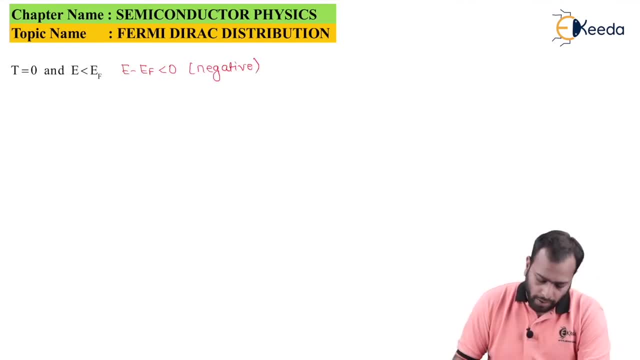 quantity. Now, considering that equation f of e is equals to 1 upon 1 plus e times e minus ef upon kt, I get the value of e minus ef as minus, and since t is zero, I get the value as minus infinity. You all know that e raised to minus infinity is nothing but as zero, because it is 1 upon e raised. 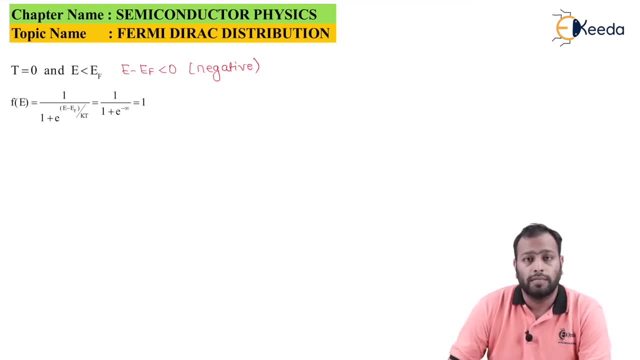 to infinity, and hence the value is 1.. What does this mean? This means that all the energy states below the Fermi states are completely filled with electrons, or I can say all the energy levels below the Fermi level are full. So if they are full, there is 100% probability of finding the electron. 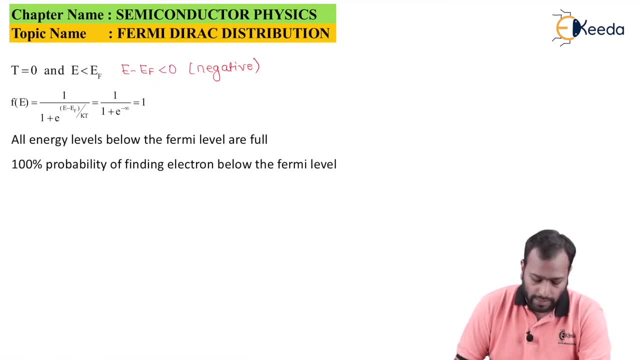 below the Fermi level. Now let's take a case where t is equal to 100% probability of finding the electron below the Fermi level. Now let's take a case where t is equal to 1 upon e raised to minus. Now let's take a reverse case, when E is equal to 0, but now E is greater than EF, which means 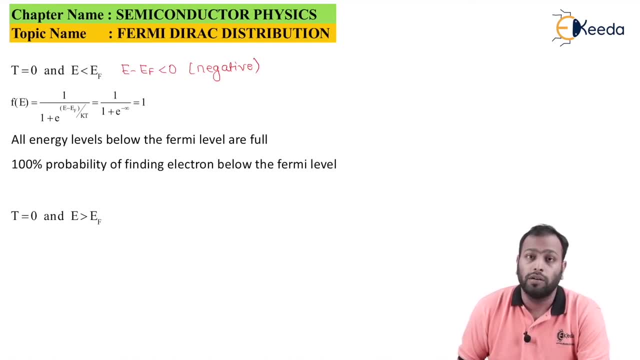 now I am concerned with that energy level which is above the Fermi level. So here I can say, my E minus EF value is greater than 0, which is nothing but a positive quantity. So again, plugging these values we'll be having, F of E is equals to 1 upon 1 plus E raised to E. 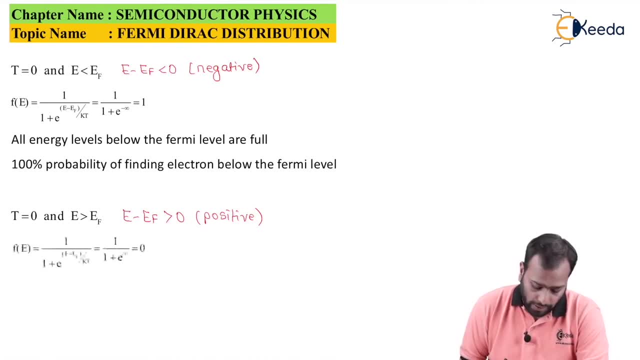 minus EF divided by kT. So here the only difference from the previous is: in this case your value will be equal to positive infinity, since the term E minus EF is greater than 0. We all know that E raised to infinity is nothing but as infinity, and 1 upon infinity will give me a probability of. 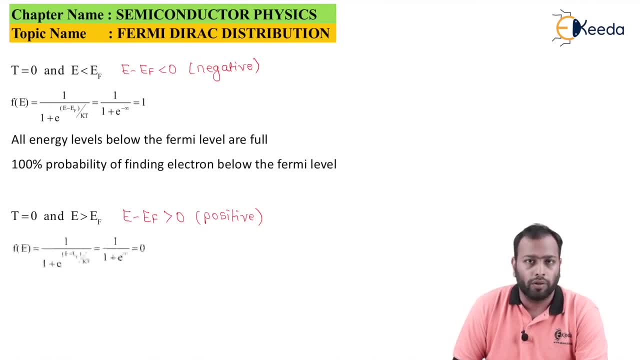 0, which means that there are no electrons found above the Fermi level. So all energy levels are equal to 0. So all energy levels above the Fermi level are empty and there is of course 0% probability of finding electrons above the Fermi level. Now let's take a third case, where E is greater than 0 and E is: